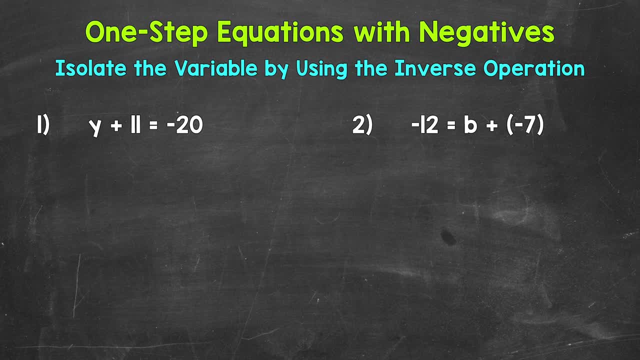 out what y equals. Since 11 is being added to y, we need to undo that addition by using the inverse operation. so the opposite operation, The opposite of addition, is subtraction. so let's subtract. Let's subtract 11 from the left side of the equation. Now, whatever we do to one side of the 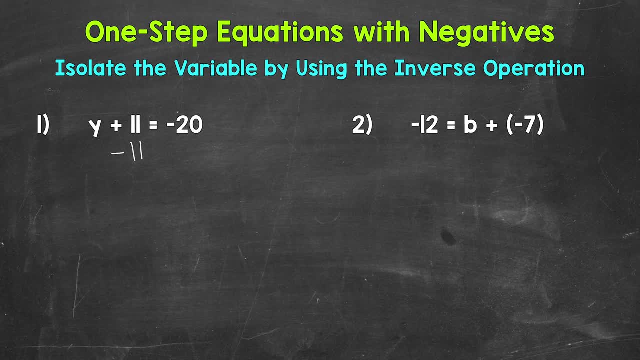 equation we must do to the other in order to keep it balanced and equal. So let's subtract 11 from the right side as well. Now, if we take a look at the left side of the equation, we are adding 11 and subtracting 11.. So these 11s cancel each other out. They equal zero. So 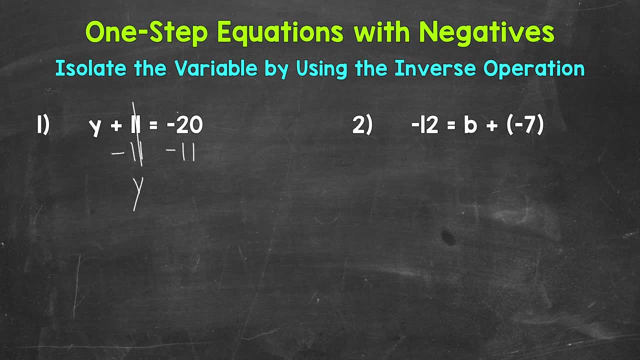 y is now isolated, It's by itself y equals. Now, on the right side of the equation, we have negative 20 minus 11.. So we're starting with negative 20 and subtracting 11.. So we are. 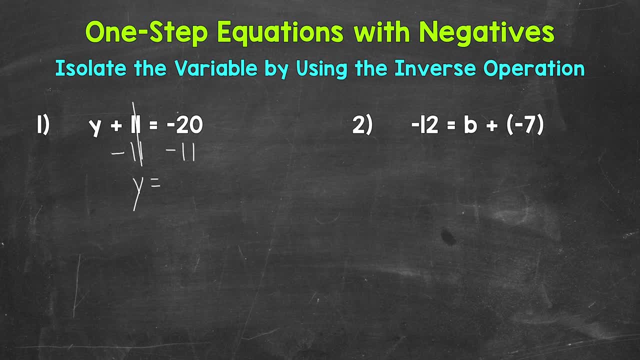 decreasing in value by 11. We end up with negative 31.. So y equals negative 31.. Now, one thing I do want to mention. it's always an option to come to the side in order to figure out a problem. For example, negative 20 minus 11, we did. 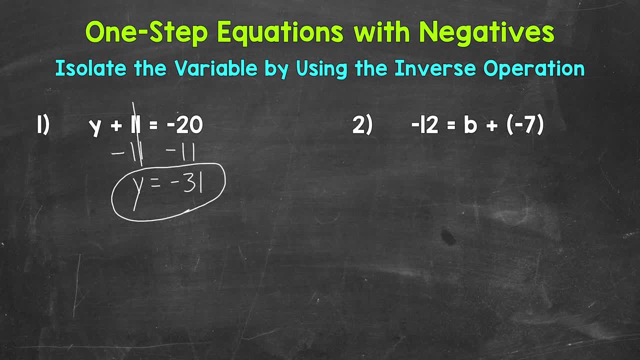 vertically. You can come to the side and rewrite this horizontally if you prefer. Now, when we subtract, we can add the opposite. So let's add the opposite here. Add the opposite. So negative 20 plus negative 11 gives us that negative 31.. So again, you can't always 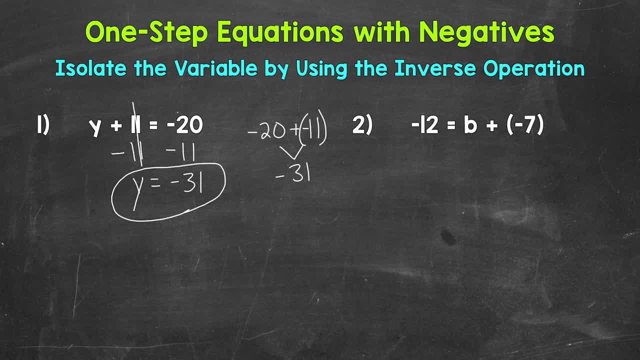 come to the side to show work or set up a problem differently. So something to keep in mind. So our solution for number one is negative 31.. We can always check a solution by plugging it into the original equation. So let's plug negative 31 in for y and see if this works. Negative 31. 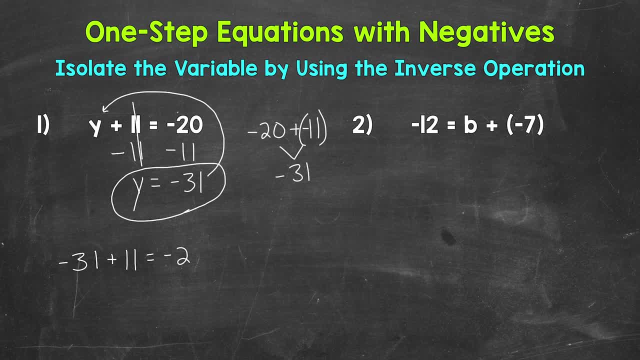 plus 11 equals negative 20.. So we're starting at negative 31 and adding 11.. So we are increasing in value by 11.. Negative 31 plus 11 does equal negative 20.. So we have the correct solution: Y equals negative 31.. 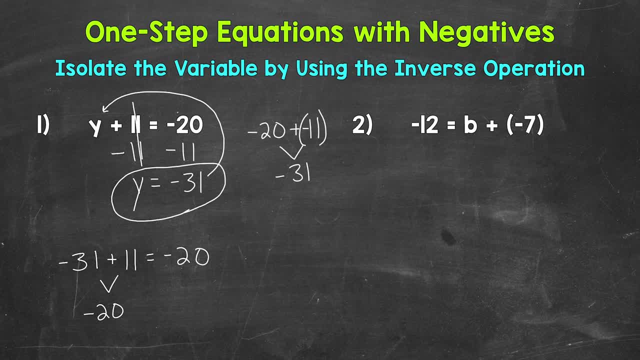 Let's move on to number two, where we have negative 12 equals B plus negative 7.. We need to isolate that variable of B. Negative 7 is being added to B, So we need to undo that addition by using the inverse operation. 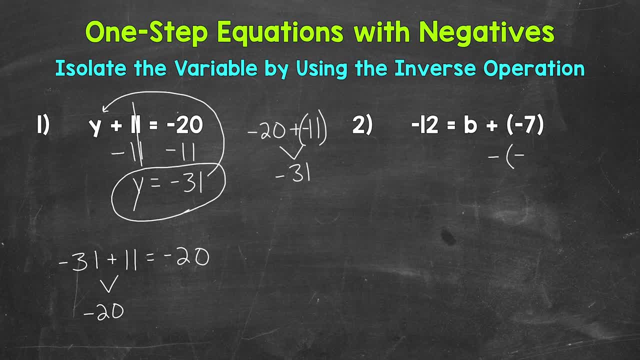 Let's subtract negative 7 from the right side. Whatever we do to one side of the equation, we must do to the other. So let's subtract negative 7 from the left side as well. Now, if we take a look at the right side of the equation, 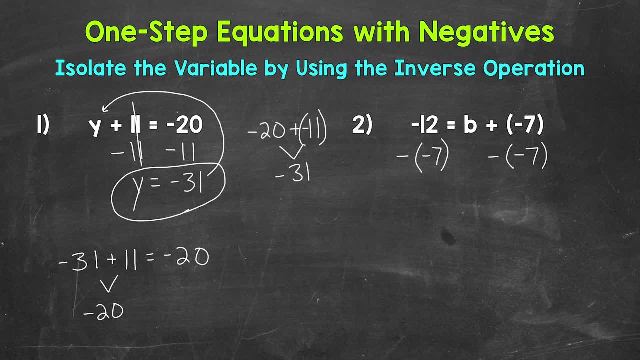 we are adding a negative 7. And subtracting a negative 7. These negative 7s are going to cancel out and equal 0. But it's kind of difficult to think through when we are subtracting a negative. When we subtract a negative, we actually increase in value. 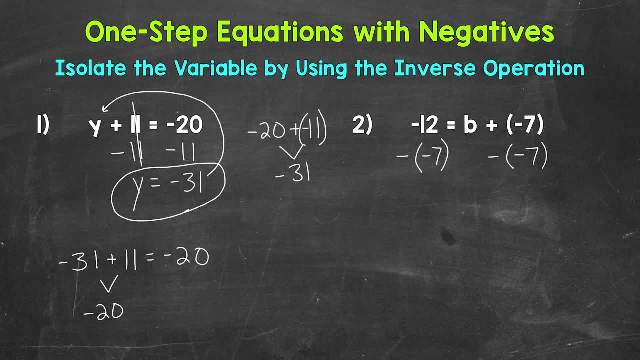 And remember, we can add the opposite. That's going to make this simpler to think through and see how the variable ends up isolated. So let's add the opposite, Add And then the opposite of negative. 7 is positive 7.. So whenever we subtract a negative, we can add a positive. 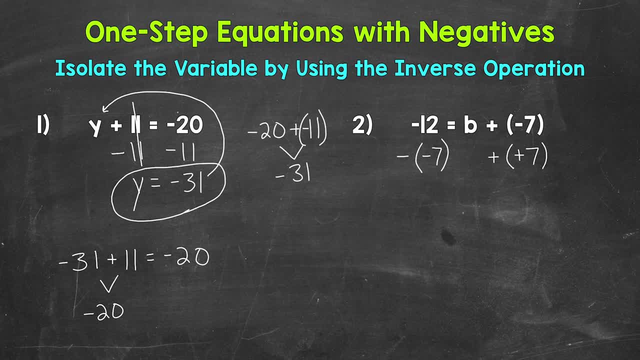 So now we have a negative 7 and a positive 7. These 7s cancel out. They equal 0. So the variable is now isolated. B equals. And then on the left side we have negative 12 minus negative 7.. 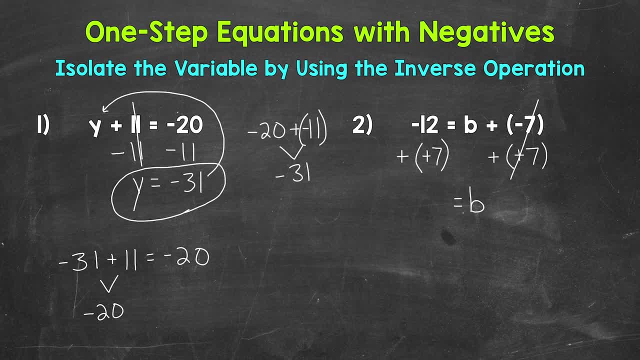 Let's add the opposite. Add The opposite: Negative 12 plus a positive 7 equals negative 5. So B equals negative 5.. We can rewrite this with the variable coming first, And remember we can always come to the side in order to show work. 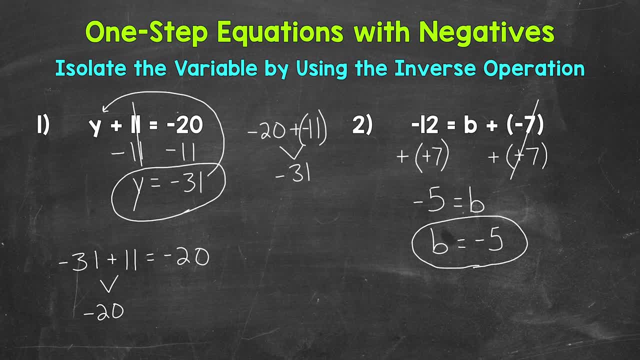 or set up a problem differently. For example, let's do negative 12.. Minus negative 7 off to the side and set it up horizontally. Let's add the opposite. So add the opposite. Negative 12 plus a positive 7 gives us negative 5..